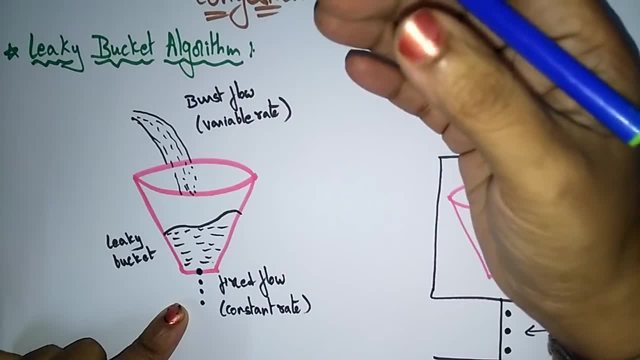 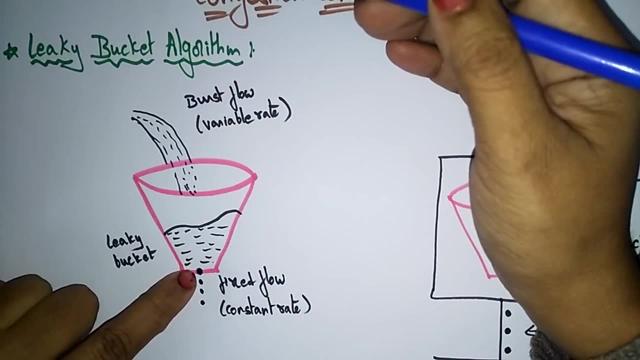 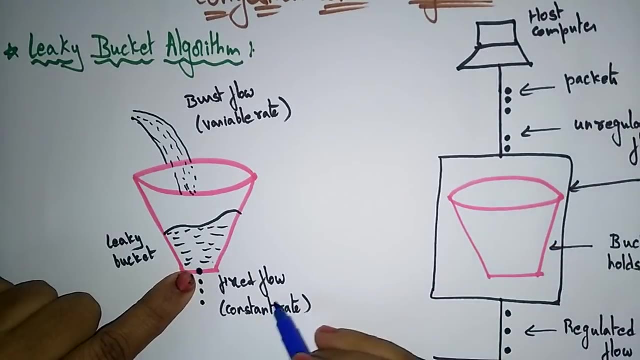 the force it is coming and how much water. it's a fast or slow, and the water rate is a, it's a, it's no matter, Okay. and the hole is a. it's a small hole, So in that hole a constant flow will be coming out. means a fixed flow. was there only drop by drop, Okay, so the outflow is at constant. 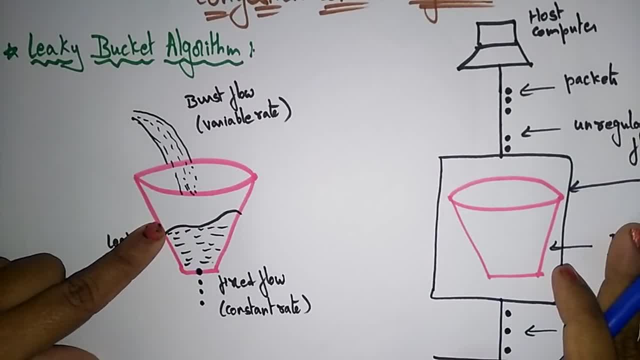 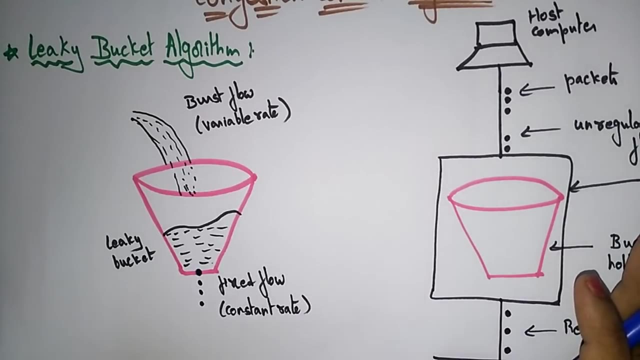 rate, Suppose when the bucket is full with water. suppose the bucket is full with water, with lot of water. what it happens? it entering into spills over the sides and is a lost because the outcome is only the fixed. It is a constant rate. only drop by drop it is coming. But if you pour lot of water the bucket is. 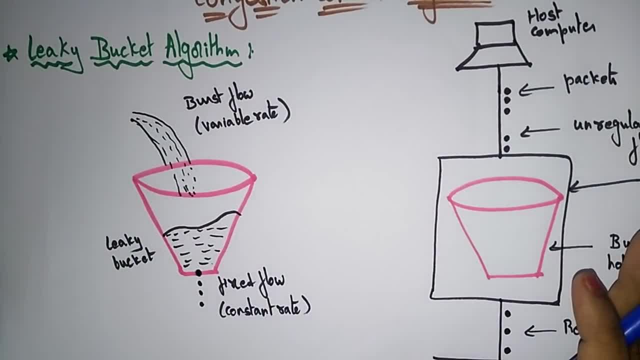 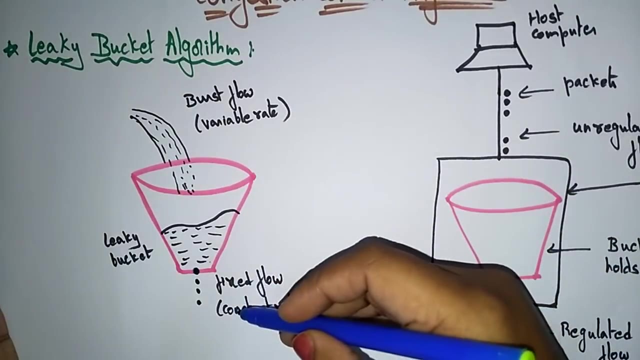 full and water completely. this filling out means spill out. Okay, so what happened? if water is spill out, the data will be lost, So means the water is wasting here. So suppose it is also coming in the constant rate. if it is going out in the constant rate it's no problem, But here it's a. 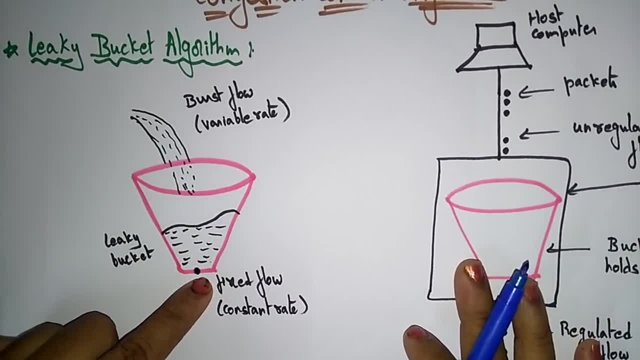 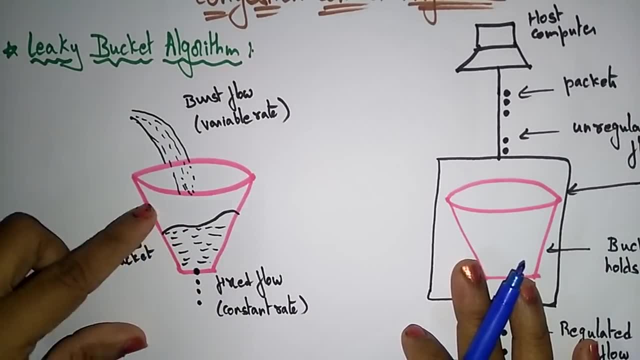 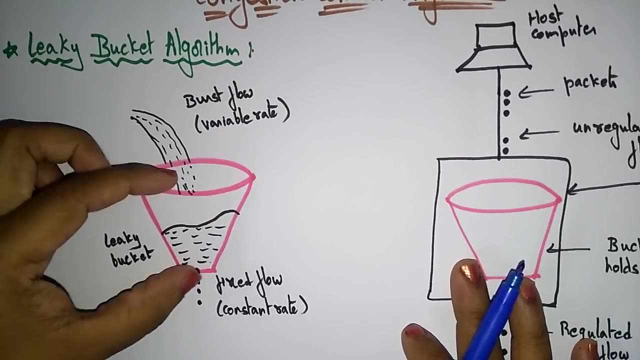 water is coming at the variable rate. Okay, Okay, Okay, Okay, Okay, Okay. Here the water is coming out, pouring in the bucket is a variable rate and coming out is a fixed rate. So whenever the overflow bucket is full, the water is spill out. So this is a general example, So same 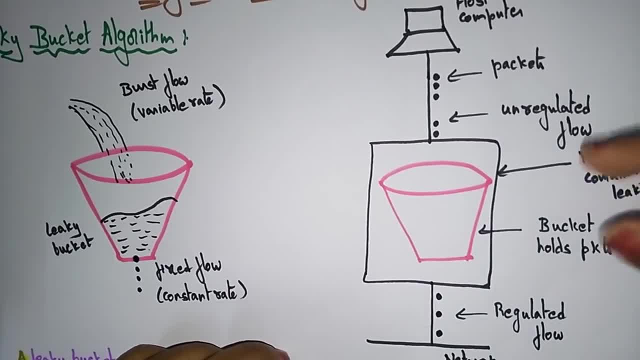 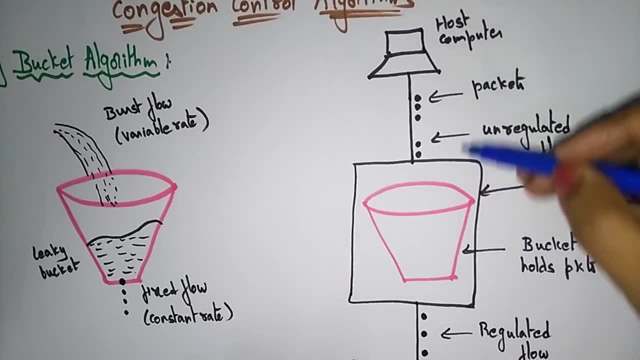 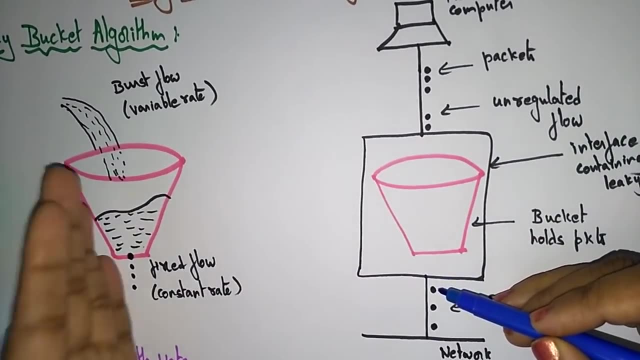 example will be taken in the terms of packets. So here is a host computer, was there, Okay, host computer. the computer is sending the packets over the network. So how it is going to be send the packets over the network. So just take this example like this: Similarly here in this, also, each network. 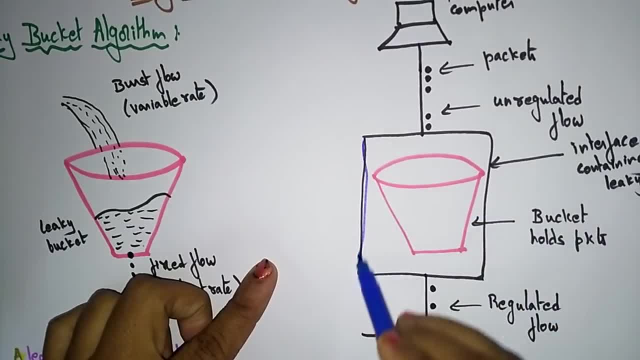 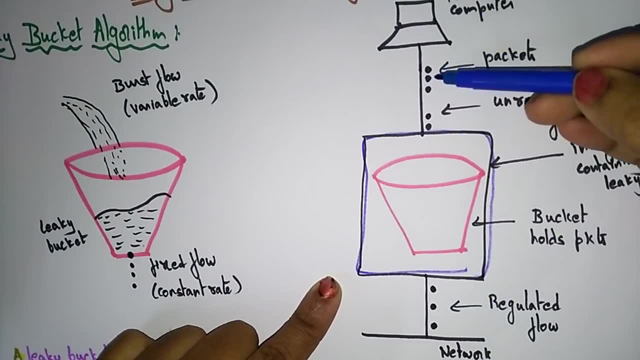 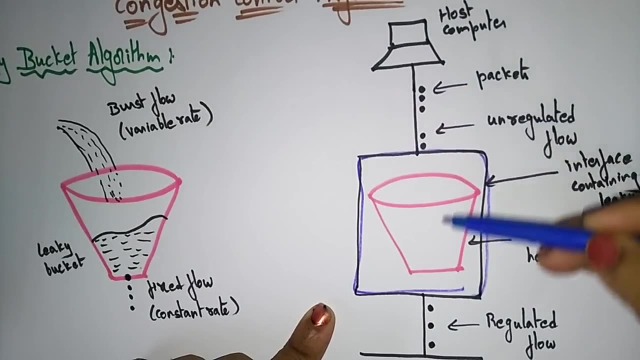 interface contains a leaky bucket, So this is a leaky bucket, Each network interface containing a leaky bucket. So when host wants to send the packets is thrown into bucket. So here the host computer is sending the packets and those are thrown into the packet bucket. So those packets 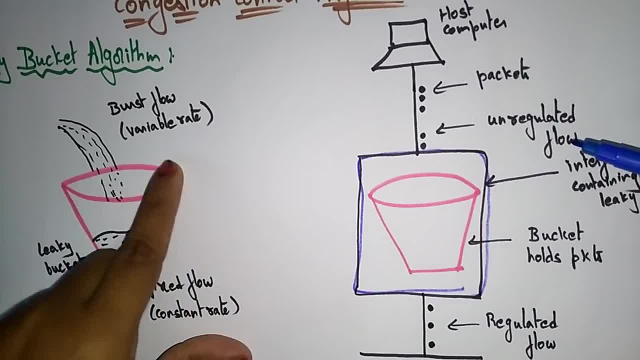 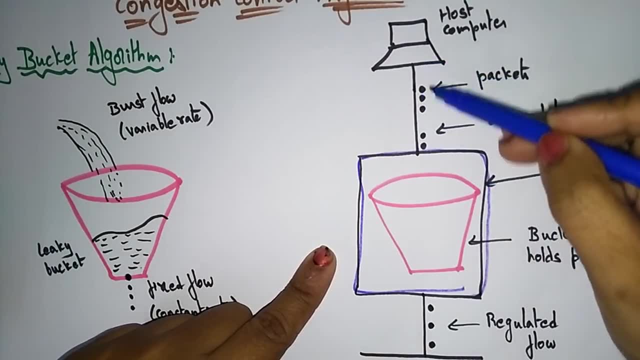 are not in a regular way. It means it's not a variable rate, unregulated flow. So some sometimes it is sending three packets, Sometimes it is sending two packets, Sometimes it's sending all the five packets. like that There is no regulated flow, it is unregulated flow.